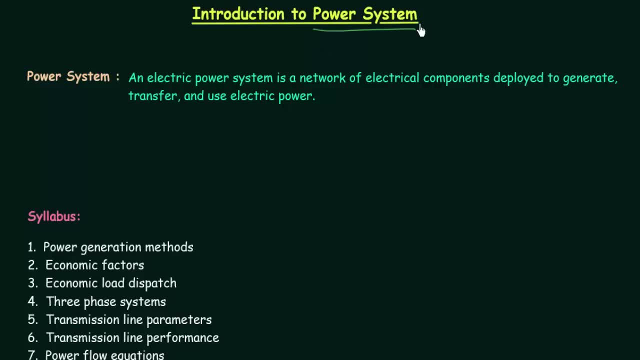 From this lecture we will start a new course: power system. This course is very important for electrical engineers. There are four to five important courses for electrical engineers and power system is one of them. There may be different names of this course. One is power system, other may be power systems or analysis of power system, and you will study this course in two different parts. In your colleges they will teach you this course in two- two different parts. 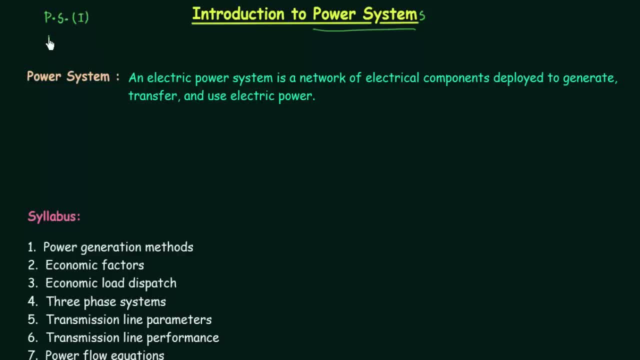 First one is power system one and second one is power system two. and if the name is analysis of power system, then the name of course will be analysis of power system part one. analysis of power system part two. In one semester you will study the first part and in the other semester you will study the second part. We will cover the entire syllabus. Syllabus of part one and syllabus of part two will be covered in this course. 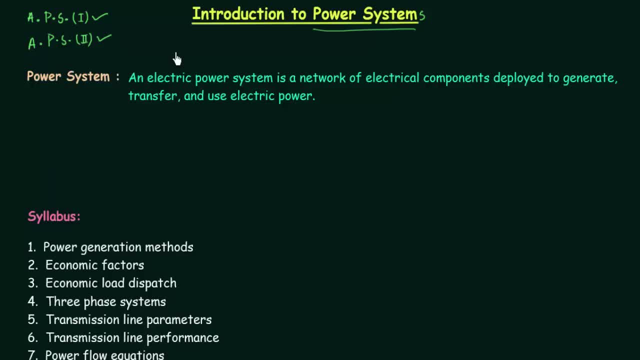 In this course, and if the name of the course is different in your college, then it is not an issue, because we will study each and every topic. and I want to make one thing clear in the beginning, and this is for Indian students. Indian students, This course is designed based on syllabus of GATE and IES. There are two important exams. The first one is GATE. 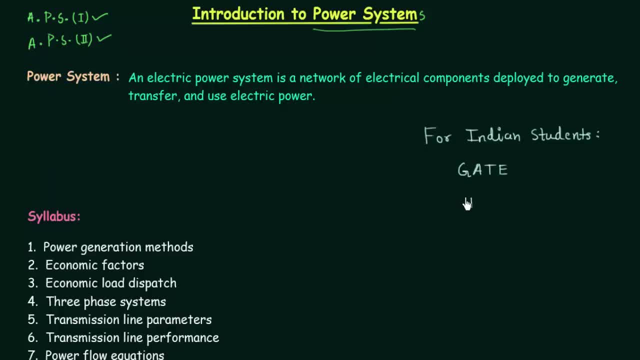 The graduate aptitude test for engineers and the second one is IES exam, and the power system we are going to study will be based on syllabus of GATE as well as IES, and if we talk about GATE then there may be 8 to 10 marks problems in your exam. Out of 100, you may get 8 to 10 marks problems from the power system, So it is 8 to 10 percent. 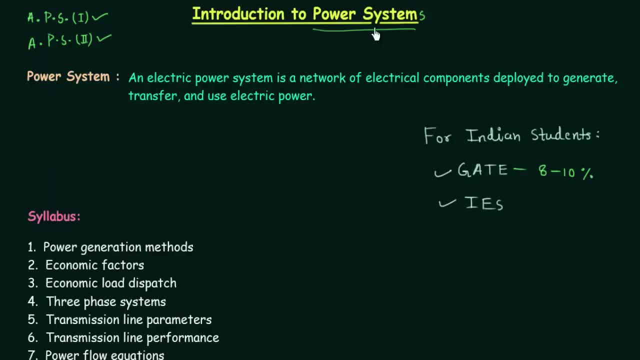 of the total syllabus. Therefore, power system is very important from GATE point of view and for IES. you may get 40 marks problem in the objective and 40 marks problem in the conventional. So for IES also, power system is very important and the course is designed based on these two exams. I will also start a new playlist. 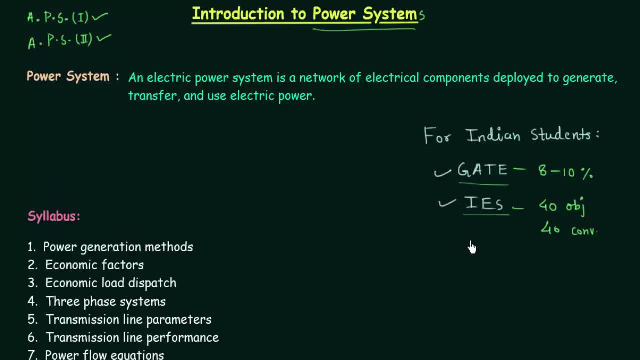 for GATE and IES solved problems, and if you are not from India and you want to understand the subject more, then you can follow that playlist. We will solve few complicated as well as conceptual problems in that playlist and, believe me, the understanding of the subject is not complete until you solve different types of problems. So, for problems, follow the playlist having the GATE and IES solved problems. and now we will start the subject. 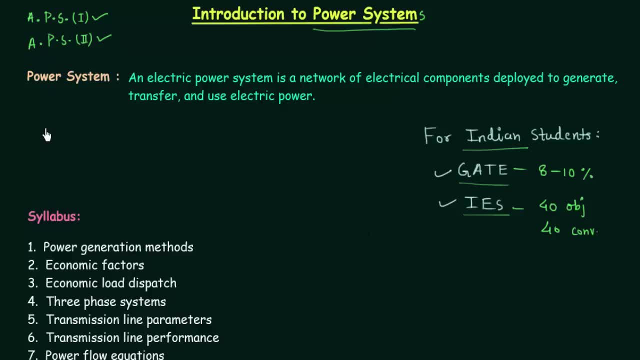 We will start the introduction to power system. The first question comes in our mind is: what is power system? So first I will read the definition, then I will explain it. and electric power system is a network of electrical components deployed to generate, transfer and use electric power. So what we can understand from here: we are generating electric power. 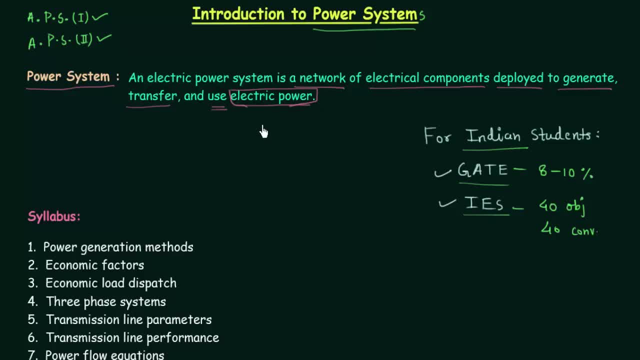 The first thing is generation of electric power, and then we are transmitting that generated electric power to longer distances. I will explain why we transmit the electric power over long distances. There is important reason behind this, and after that we use the electric power. We distribute the electric power to the power source. 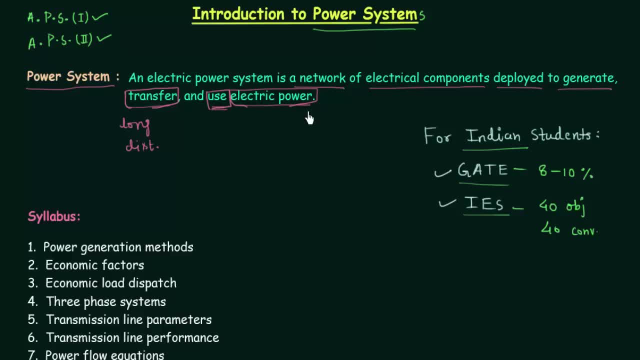 We distribute the electric power to our houses, and there we use the electric power to run different electrical equipments. So this is the task of power system. We can divide the task into three different parts. I will write them down. The first one is generation: The generation of electric power. Then the transmission of electric power: Transmission of electric power over long distances. After that distribution of electric power. 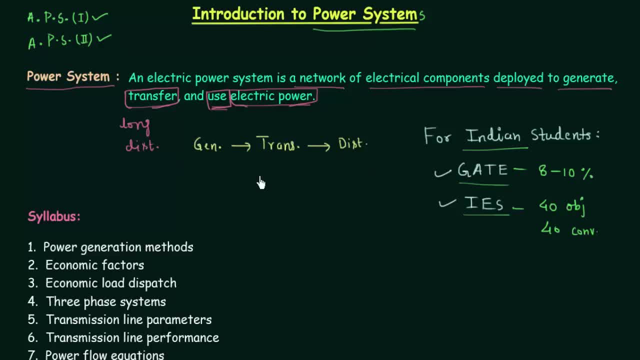 Of the transmitted power. So generation, transmission and distribution is what we have to study in this course and we should carry out this three efficiently. The process must be efficient because we want the cost to be minimum. We want to supply the electric power having the minimum cost to the consumers. Consumers are important and we want to satisfy them, and they will be satisfied only when the electric power is supplied. 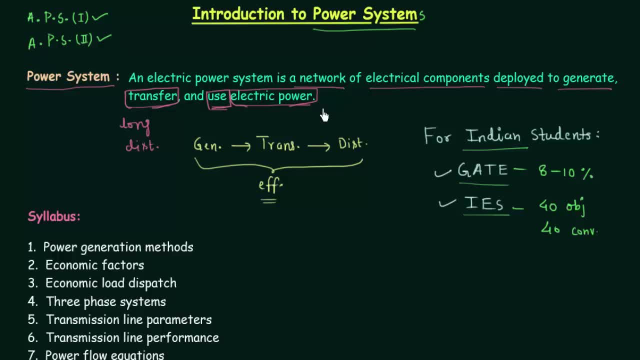 Electric power they are getting is cheap. So for cheaper electric power, these three processes must be efficient. So this is what we are going to study in this course and, regarding the generation, I will explain how the electric power is generated using different methods, In that we will study thermal power plant, nuclear power plant, hydro power plant and a few other power plants. These three power plants are very important: Thermal, hydro and nuclear. 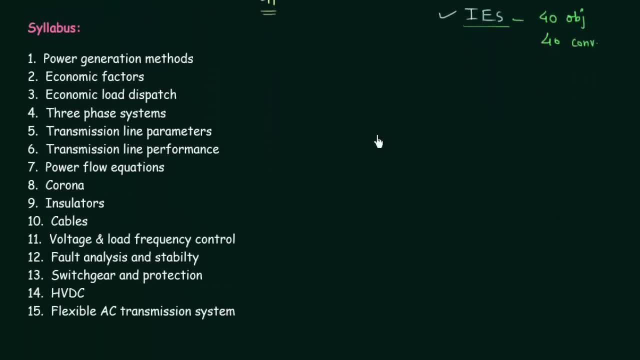 Now you may note down the syllabus of the course. The first part is the power generation methods. I told you we have different power generation methods. The first one and the most popular one is thermal, and I am talking about India. In India, the major power supply is from the thermal power plants. Thermal means we are burning coal or any other fuel to generate power. 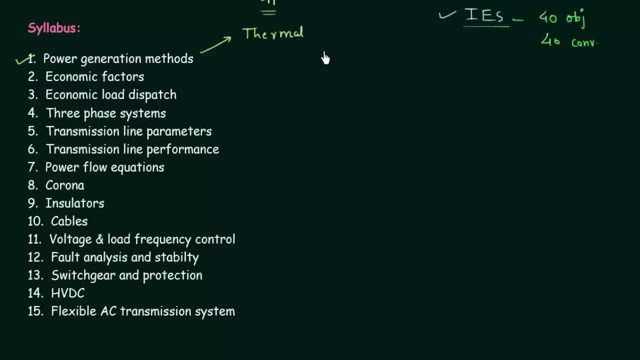 To heat the water in the boiler so that steam is produced, and that steam is used to run the turbine, and the generator is connected to the turbine with the help of prime mover and then the electricity is produced. In India, 70% of the total power produced is from the thermal power plants. After this we have hydro power stations. In hydro power stations we use the potential energy of stored water to generate power. 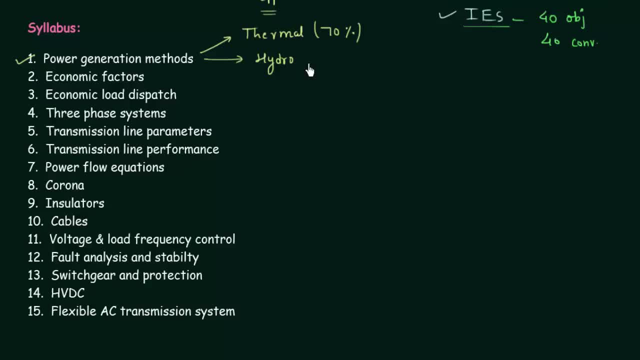 We construct dams and the stored water is then used to run the turbine and electricity is produced. 20% is from hydro. Then we have nuclear. Nuclear is similar to thermal, but instead of using coal we use the nuclear fission. the heat released from the nuclear fission to heat the water and convert it to steam. 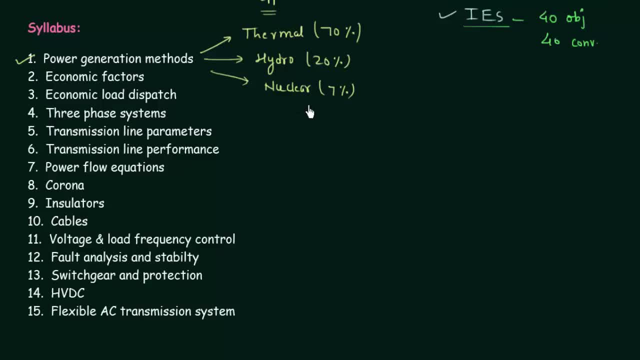 And 7% is from the thermal power plants, Nuclear. So how many is remaining? 3% is remaining, So 3% we obtain from other sources like wind, sun or you can say solar, etc. So this is what we are going to study in power generation methods. After that we will study economic factors. This is very important. As I already told you, the electrical power must be cheaper, and for that we have to consider renewable energy. 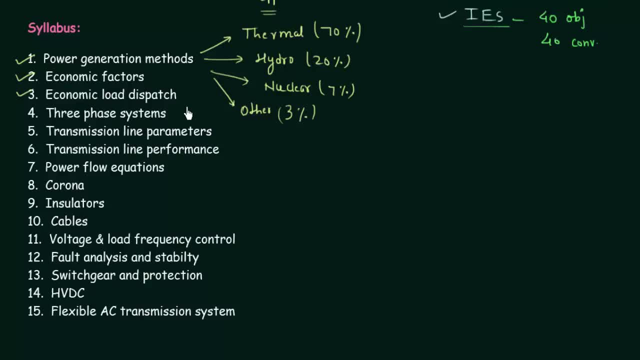 Various factors. Then we will study economic load dispatch. This is another important topic And these two topics are important and easy and you will have problems in your exam. So try to focus on these two topics because they are pretty easy and you can easily solve problems from these two topics. 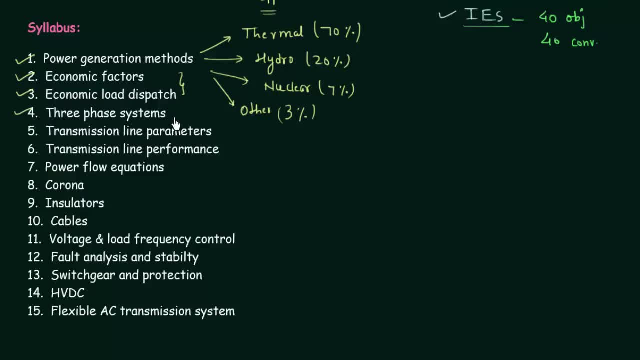 The fourth one is three phase systems, Again important topic. We will understand what are three phase systems. After this we will study transmission line parameters. These three parameters are transmission line parameters. Then we will understand the line performance, That is, the transmission line performance. 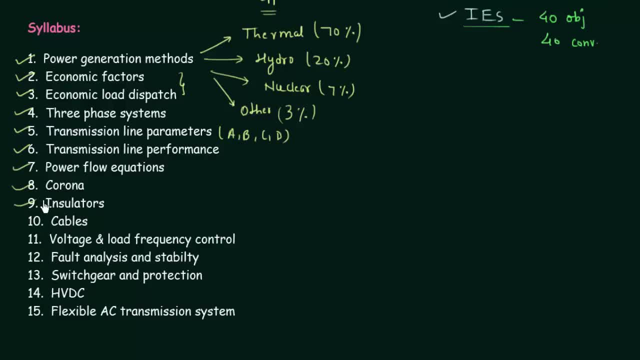 Power flow equations, Corona Insulators, Cables, Voltage and load frequency control. Twelfth one is fault analysis and stability. Thirteenth, switch gear and protection. Fourteenth, HVDC- High voltage, DC transmission. Regarding this, Keep in your mind, whenever the distance is long, then we use HVDC instead of HVAC. Instead of transmitting the AC power, we transmit the DC power. This is more economical for the longer distances. 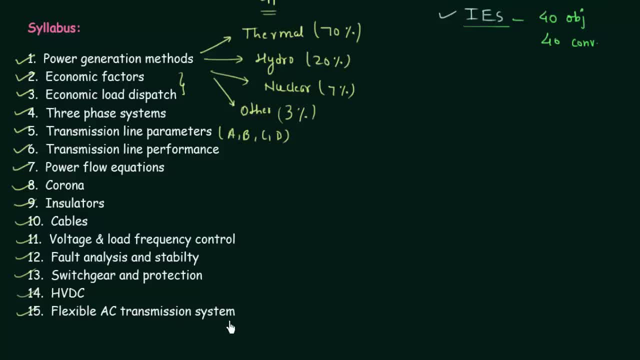 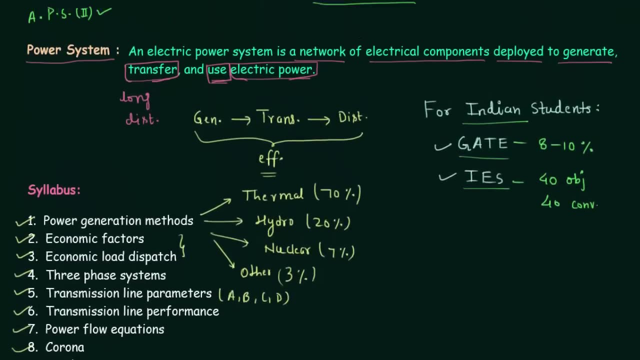 Fifteenth one is flexible AC transmission system. Under this we will study various devices to improve the performance of power system. In short, We call it FAC transmission. After this I will explain various objectives of power system. This is the most important part of this lecture. 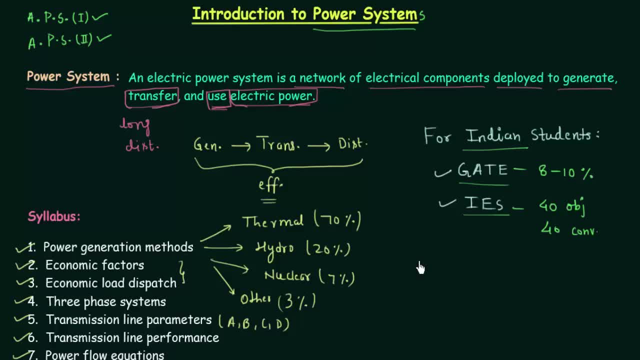 We will try to understand what are the objectives of power system and based on those objectives you can divide the syllabus. The objective number one: the objective number one is the cost. We want the cost of the electrical power to be minimum. The first one is: the cost of electrical energy must be minimum. 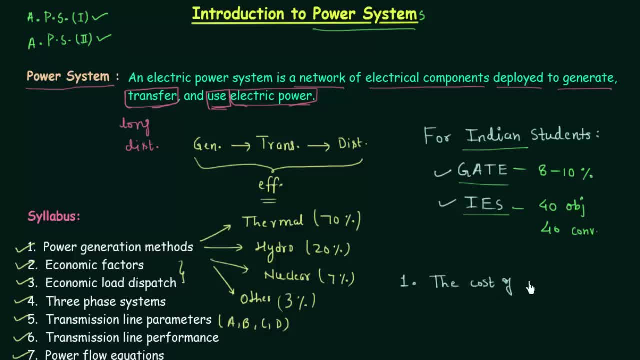 I will write this down: The cost of electrical energy must be, must be minimum, And this is the first point, or you can say first objective of objective of power system. So this is the topic and under this we will study economic factors. 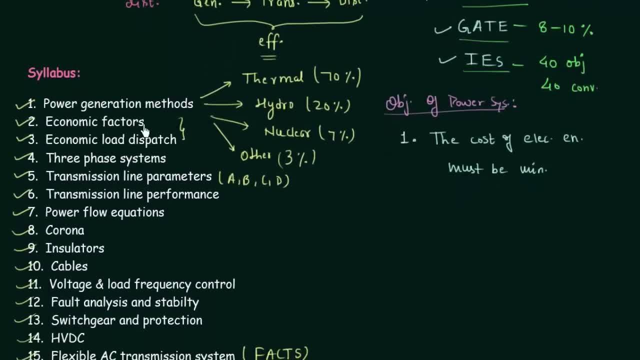 You can see the second point in the syllabus. It is economic factors. So we will study economic factors. After this, we will study economic load dispatch. Economic load dispatch, Economic load dispatch- Okay, Economic load dispatch. And the third one is generation. 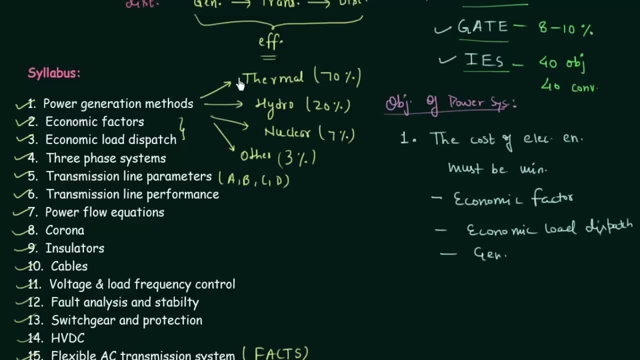 We will also try to understand how we carry out generation in thermal, hydro, nuclear and other sources of power generation. You will get how the different actions in this power plants are related to cost cutting. The second objective is we want to supply rated voltage and frequency to the consumers. 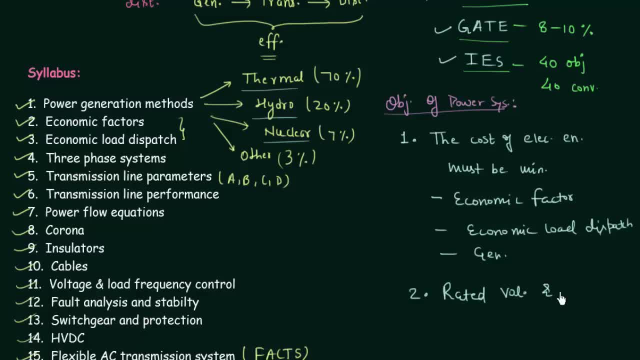 So rated voltage. Now, when we start with rated voltage and frequency, we want to supply to the consumers And for this we will study voltage control and load frequency control. voltage and load frequency control: This is very important topic And in this syllabus you can see the 11th point: voltage and load frequency control. 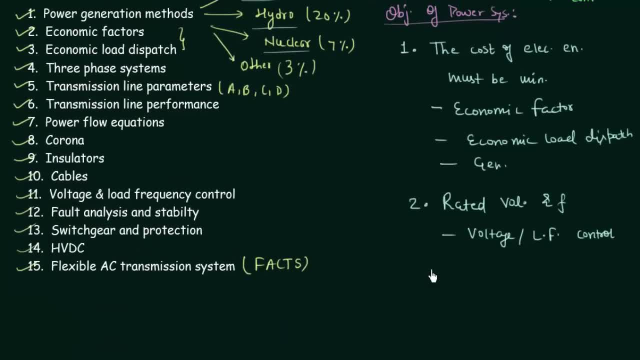 The third objective of power system. It is Is Is power supply. We want to provide reliable and continuous power supply to the consumers. I will write this down: Reliable and continuous power supply. This is very important because no one likes power cuts. The power should be reliable and it should be continuous, and for this we will. 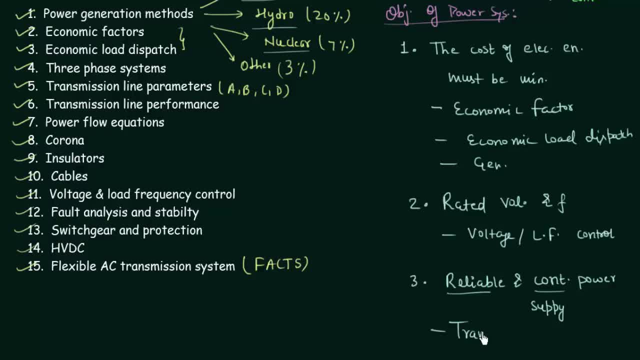 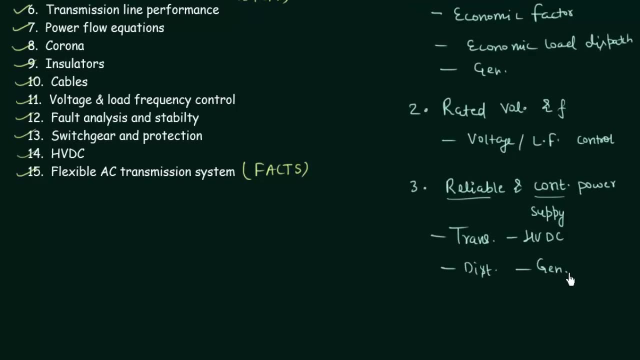 study transmission: part of the syllabus transmission part of the syllabus: HVDC high voltage DC transmission. We will also study distribution, distribution and generation in this part, The fourth objective. the fourth objective is to have most efficient and faster fault clearing equipment- There are faults in power system- and to clear the system. 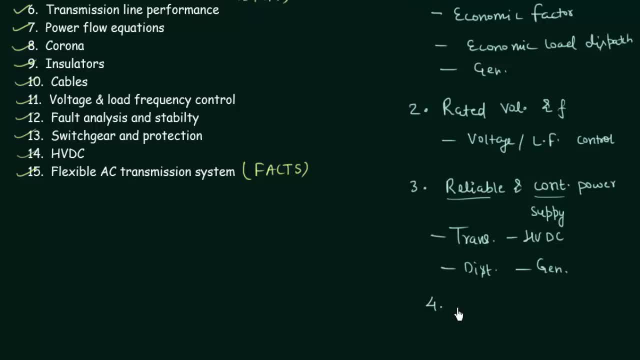 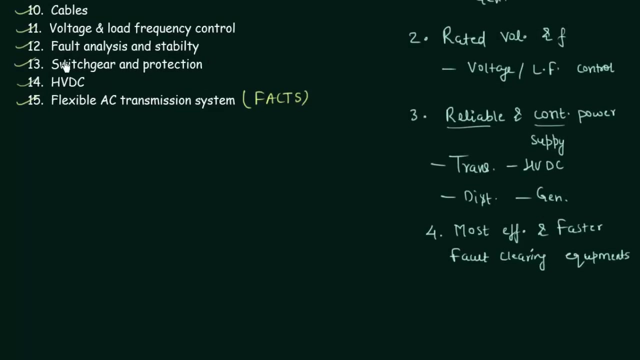 most faults. This means to isolate this fault from the healthy system. we need more efficient and faster fault clearing equipments. I will write the fourth objective: Most efficient and faster fault clearing equipment, Equipments- Equipments This equipment should have- best we will use to clear the fault or you can say to separate the faulty section from the healthy system. and for this we will study fault analysis and switch gear and protection. Fault analysis, this one, and switch gear and protection. 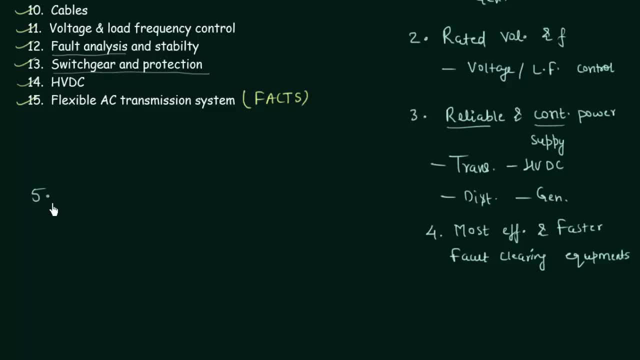 The fifth objective, I will write down stability of generator. We know what are faults. Faults occur in the line and the fault are generally temporary. For example, a tree touching the overhead lines and when the wind blows in the opposite direction, the tree will not touch the line. 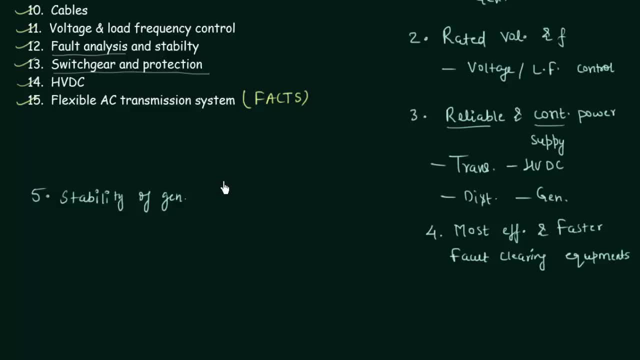 So the fault is temporary and for that we will study fault analysis For that temporary fault, if the generator is losing the synchronism, then it is not good for the power system. So what I mean by the fifth objective is that most of the practical faults are temporary and due to this fault. if the generator is losing the synchronism then this is not good for the power system. 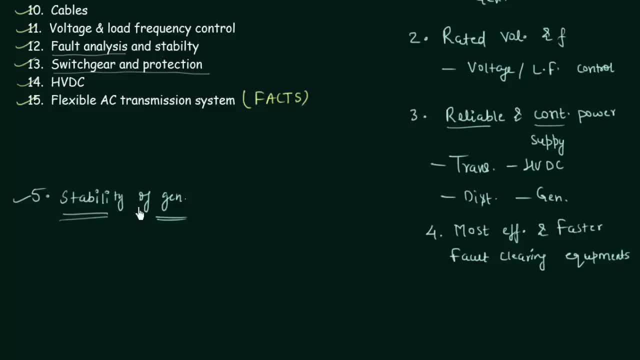 So generator must be stable. The stability of generator is very important and it should not depend on the power system, The nearer or away faults. for example, at the generating end the power is stepped up. and if there is any fault which is nearer to the generator and it goes out of synchronism, then it is not good. and if there is fault more than 400 or 500 kilometers away from the generating station and then also generator is losing the synchronism, it is not good. 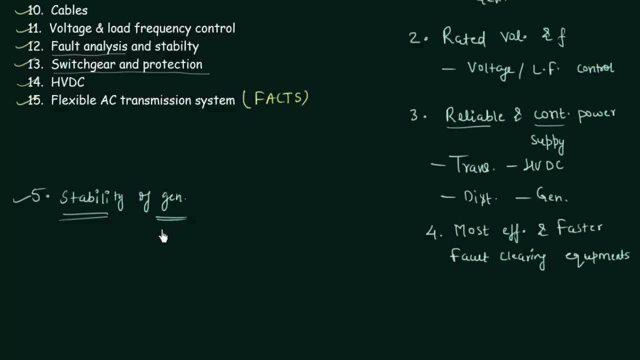 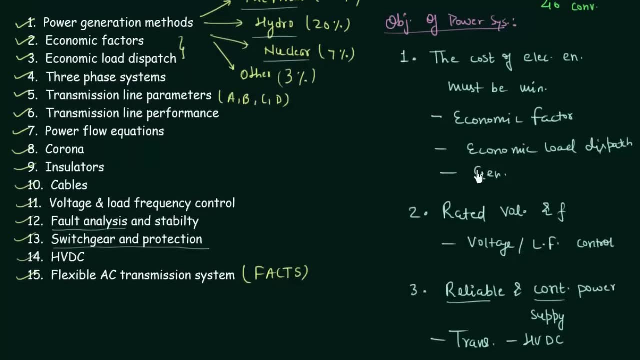 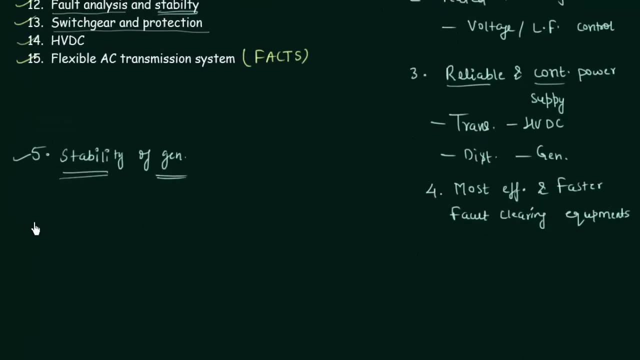 So for longer and shorter distance faults, the generator must be stable, and for this we will study Stability. in the syllabus you can see the 12th point. we have stability here, so we will study stability. the sixth and the last objective is to provide flexible power transfer over wide range of voltage and power levels, and in this we will study power cables.